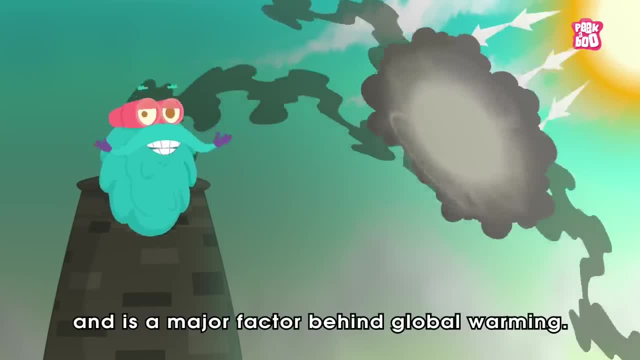 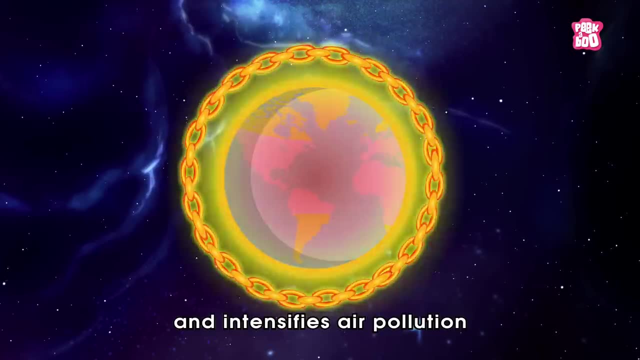 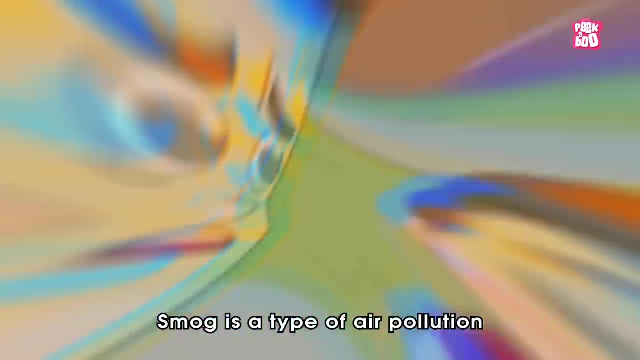 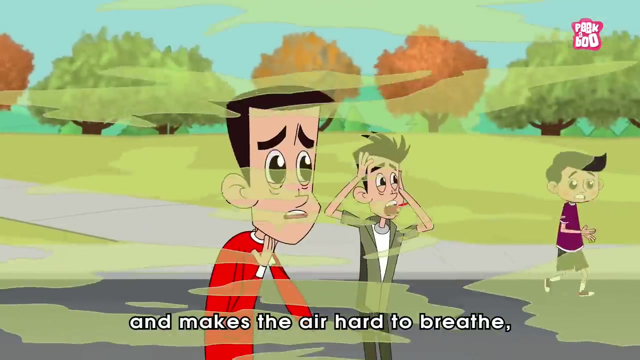 and is a major factor behind global warming. This rise in temperature sets a chain of events and intensifies air pollution by increasing the level of smog in the environment. Smog is a type of air pollution that reduces visibility and makes the air hard to breathe. 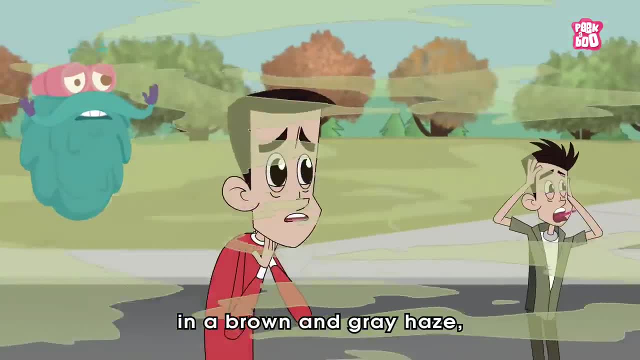 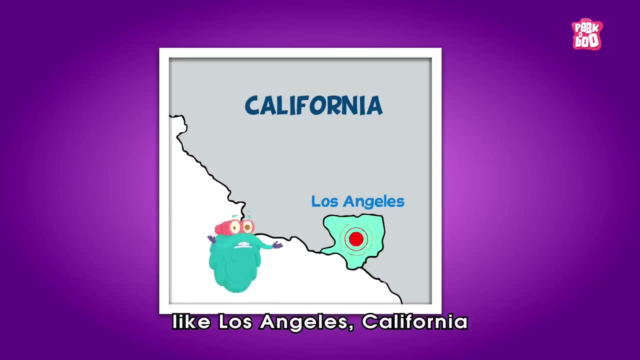 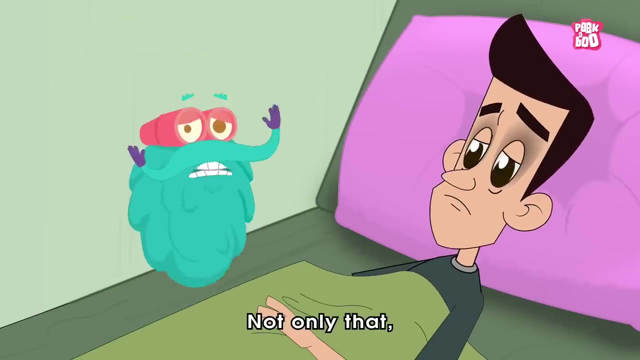 It engulfs the surrounding in a brown and grey haze, which is common in industrial areas and remains a familiar sight in cities like Los Angeles, California and Delhi. Not only that, but air pollution can also make people very sick. 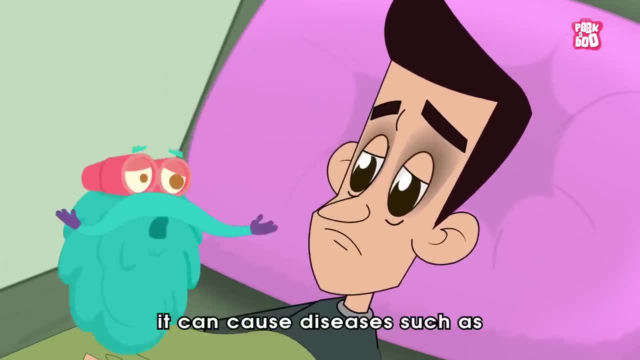 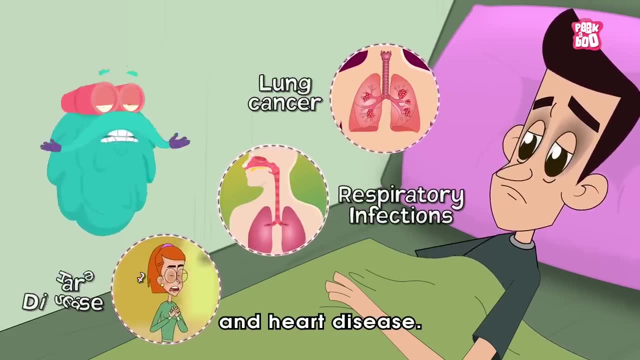 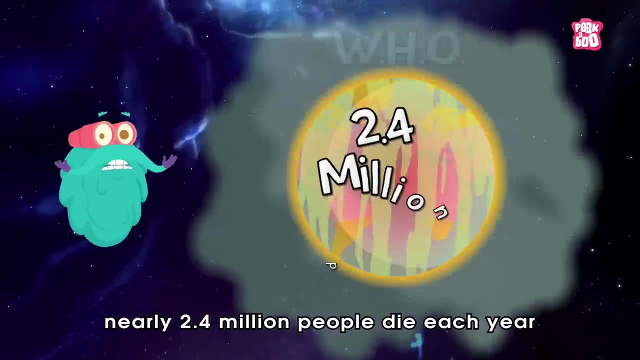 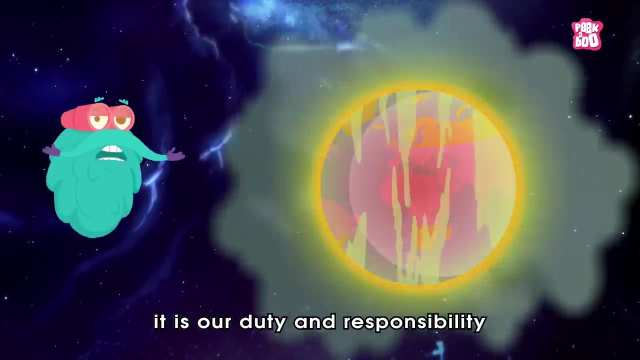 Apart from breathing issues, it can cause diseases such as lung cancer, respiratory infections and heart disease. You won't believe it, but according to the WHO, nearly 2.4 million people die each year from air pollution. So, my dear friends, it is our duty and responsibility. 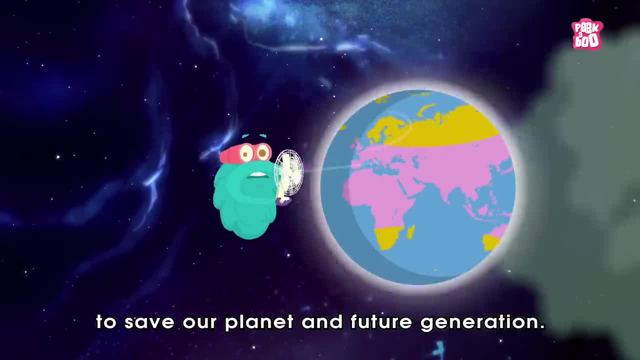 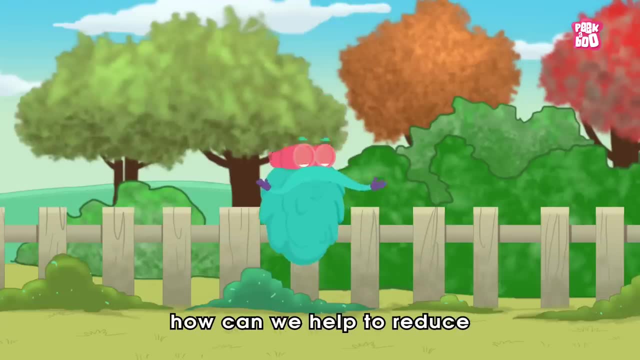 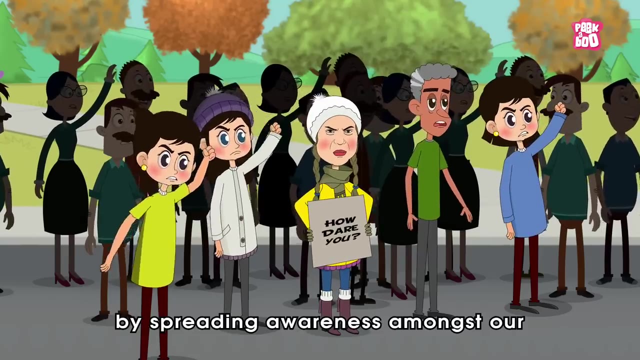 to take the matter in our hands to save our planet and future generations. But the most crucial question is: how can we help to reduce the ever increasing air pollution? Well, we can do that by spreading awareness amongst our friends and family. 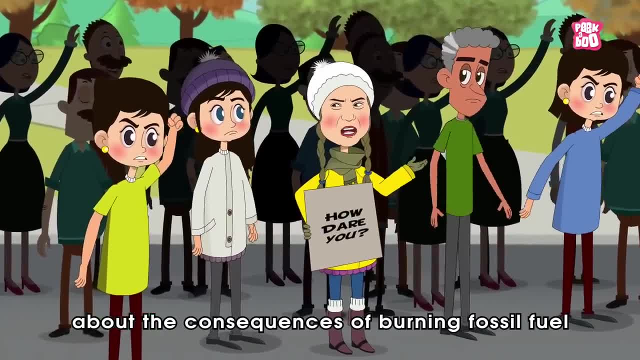 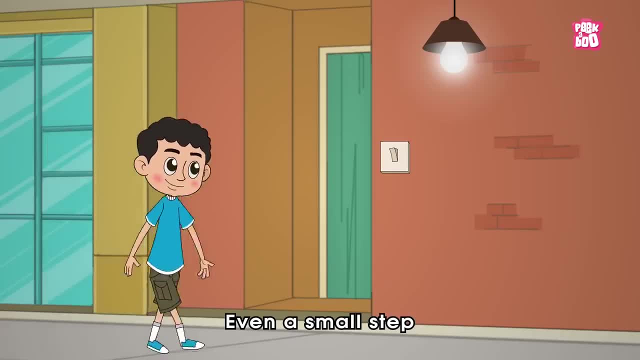 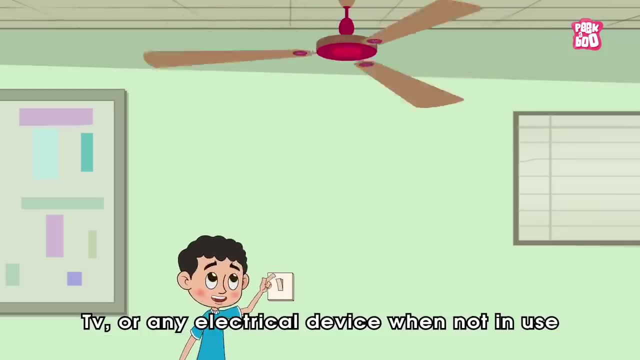 about the consequences of burning fossil fuel and urge them to reduce its usage as much as possible. Even a small step, such as switching off the lights, TV or any electrical device when not in use, can help in reducing the level of air pollution. 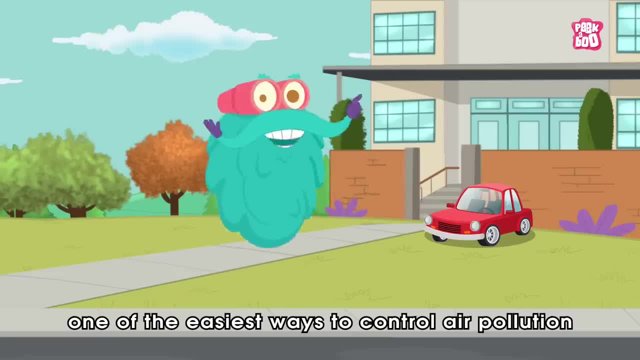 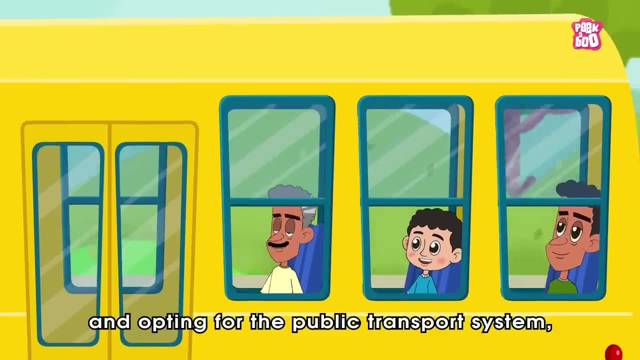 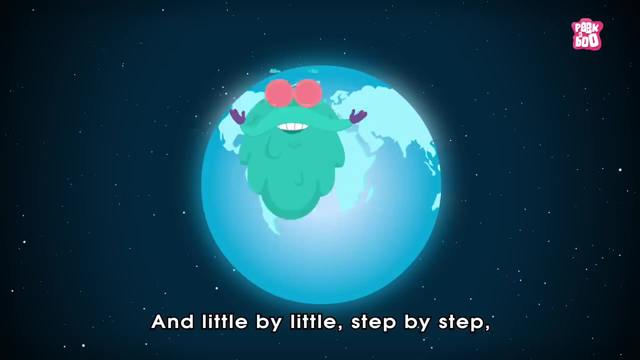 Also, one of the easiest ways to control air pollution is by limiting the use of private cars and vehicles and opting for the public transport system or walking or riding a bicycle whenever possible. And little by little, step by step, we will start to see the difference.